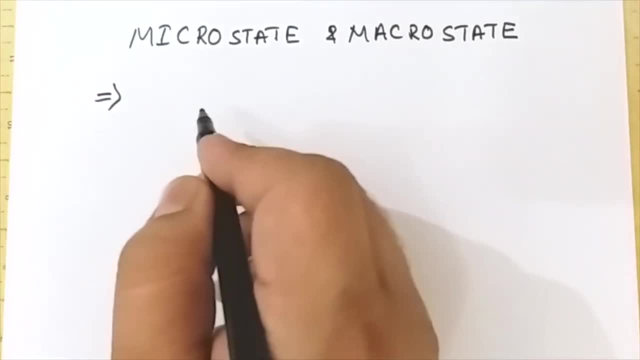 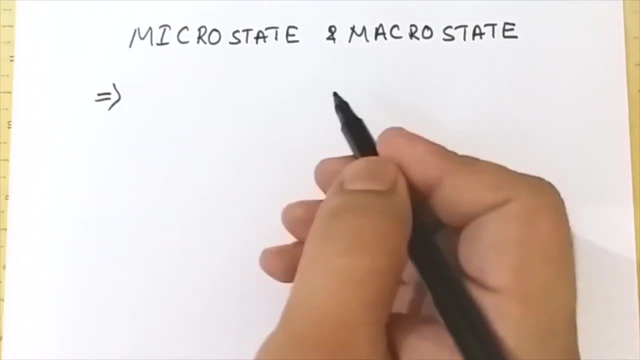 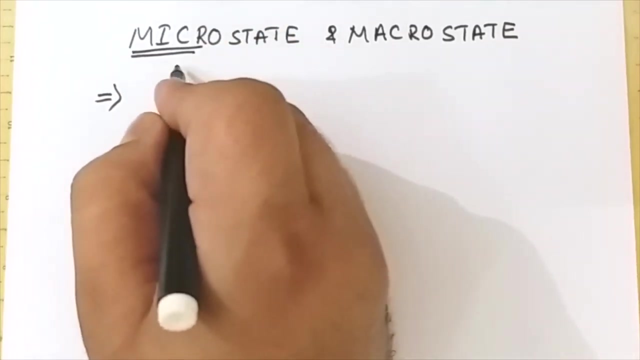 phase space and this phase space is divided into large number of cells. now, all the particles, they are present in specific cells. so microstates, they are nothing, but they are the particles that are present in that, in that phase space or in the cell. so microstates are nothing, but they are the. 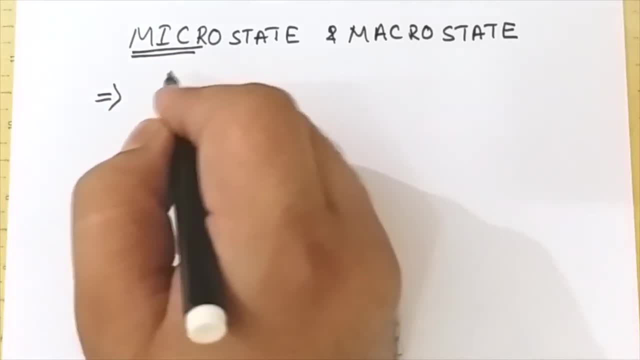 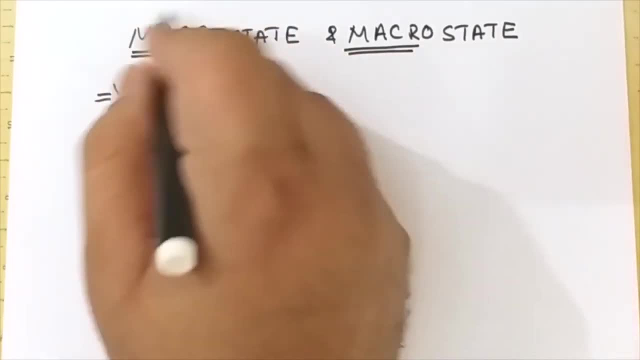 are present in the cell and the total properties that are present in the cell. and the total properties that are present in the cell and the total properties that are related to or the properties because of these particles which are present in the phase space or in the cell are known as macrostate. so 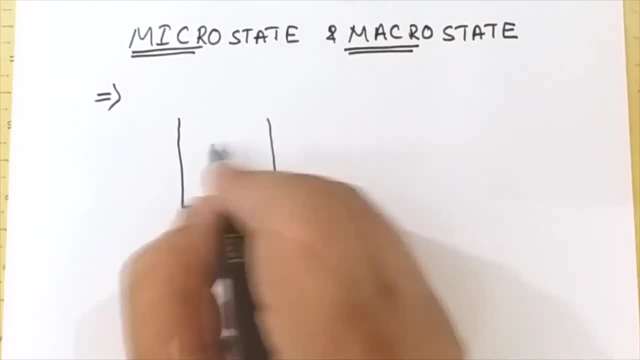 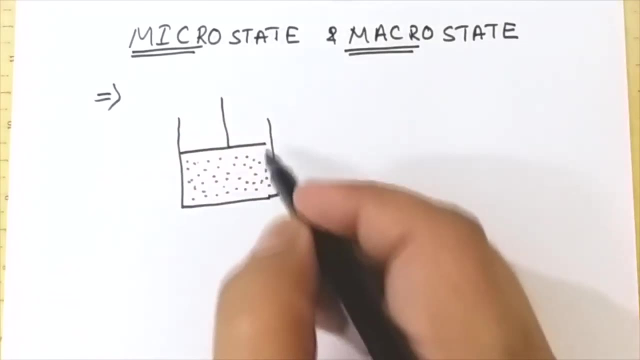 suppose, as we have seen, or suppose- let me take one example- that suppose we are having a cylinder and in that cylinder a gas is filled. now, as we know that the gas consists of large number of particles, and these particles, they are continuously in motion. so the energy, the moment. 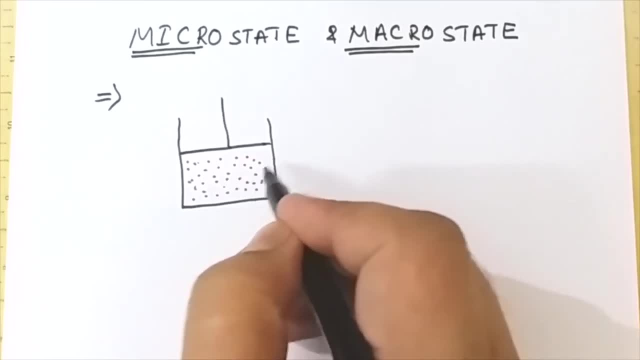 of and these particles. they are always colliding. so the energy as well as the momentum of the particle is continuously changing and the position of the particles is also continuously changing. so we can say that they are giving different arrangements at different amount of time. so this arrangement or these particles are nothing, but they are referred as microstates and 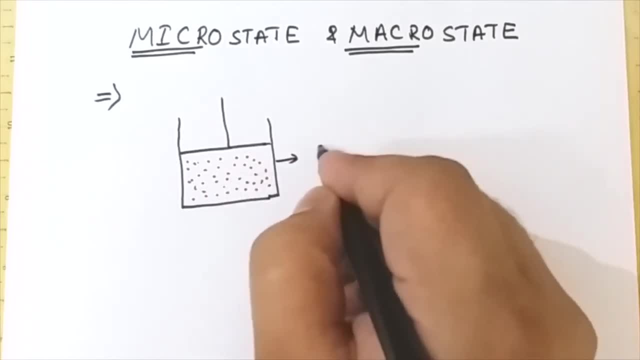 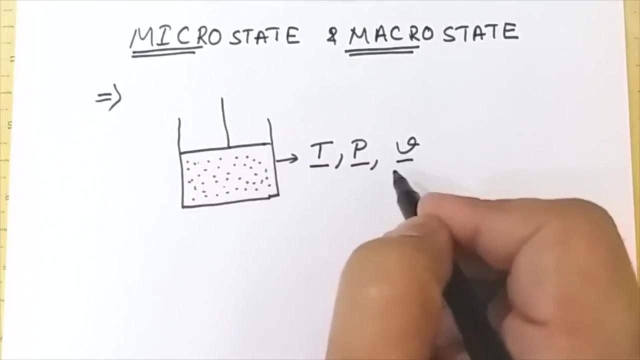 the properties due to this particle, like we can say temperature, or we can say pressure, or we can say volume. irrespective of the arrangement of the particles, the temperature, pressure and the volume of the system remains same, and hence these properties are known as macrostate of the system. 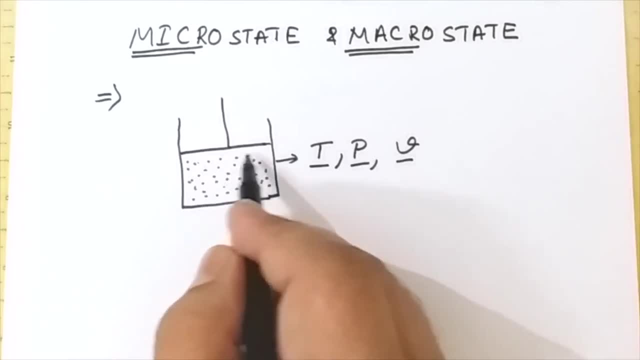 so microstates are nothing, but they are the different arrangements of the particle in the space, or we can say in the piston, and the properties which are because of the arrangement of the particles is known as macrostate. let us understand by taking one more example. nowadays there is a game which is played very much and 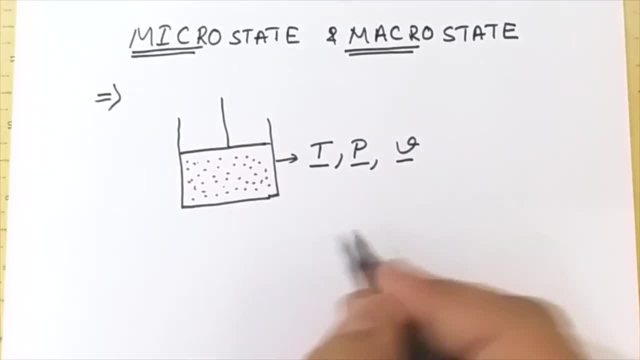 that is ludo, and in ludo two dice are thrown in order to get the sum of the dice. so suppose, if i throw a die, if i throw a die and in order to get number five, the possible combinations would be: i should get two plus three. so in order to get the sum five, the total possibilities are: 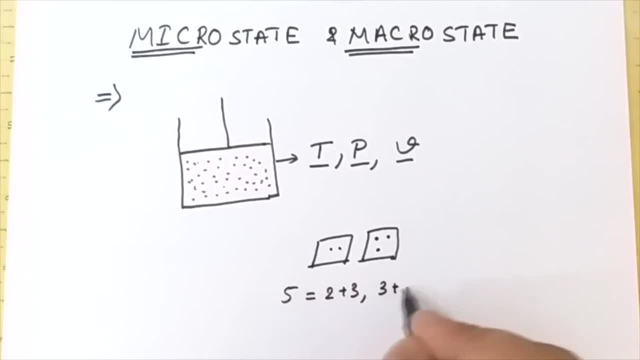 either i should get two plus three, or it should be three plus two, or it should be four plus one, or it should be one plus four. so these are the four possibilities by getting, or these are the four possibilities by which i can get the total, or some five. okay, 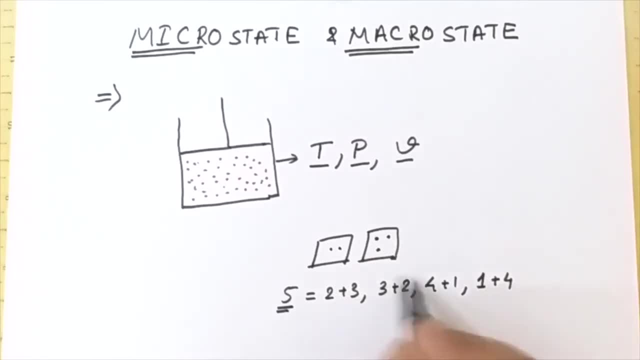 so over here, irrespective of the internal arrangement, the outer arrangement remains the same. okay, suppose i am getting four plus one, that will also be equal to five. if i get three plus two, it will also be five. two plus three, it will also be five. so this internal arrangement is nothing, but it is our micro state and the sum which we are getting. 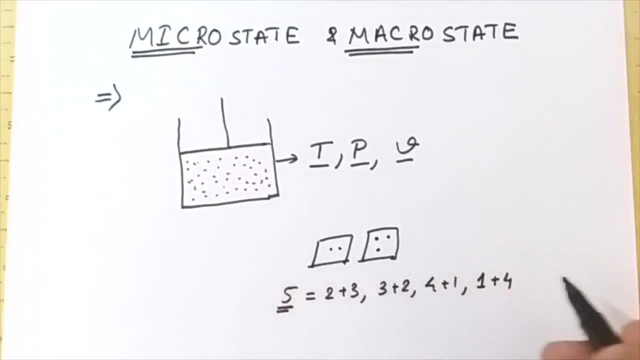 or the outer property which we are getting is our macro state. one more example: if i want seven, then i can obtain seven by either i can say six plus one, or i can say it can be five plus two, or either it can be four plus three or three plus four, or i can say 2 plus 5, or i can say 1 plus 6. 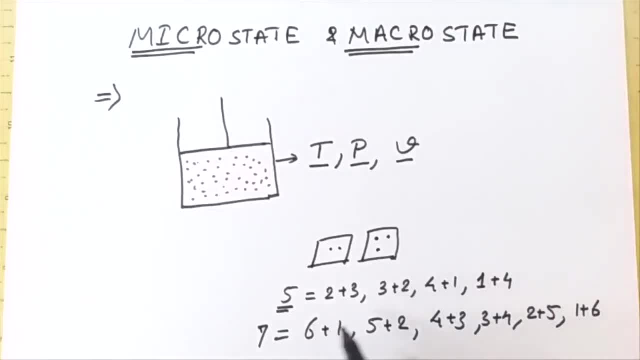 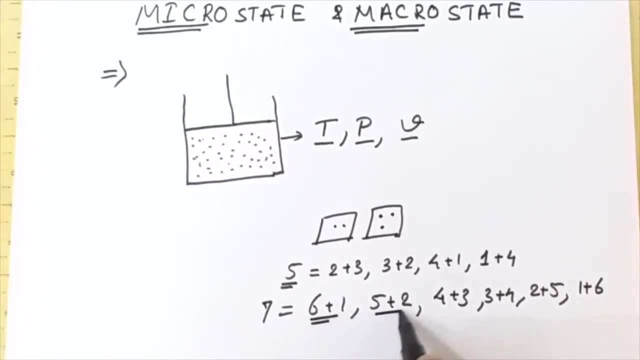 so these are the six methods. by throwing two plus three, so, and the end, either the return of the total dice, i can get the total sum seven. so over here, also again, this, this is our microstate, this is our microstate state, this is our microstate and, irrespective of the change in our microstate, our 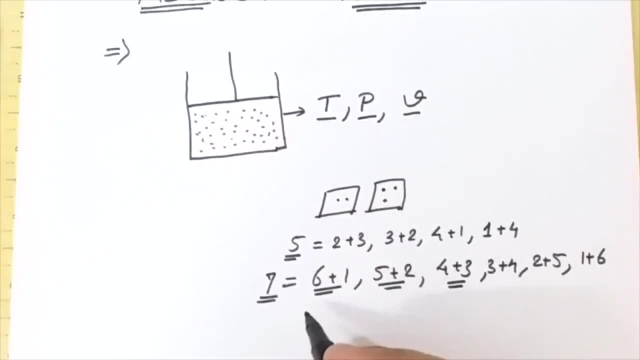 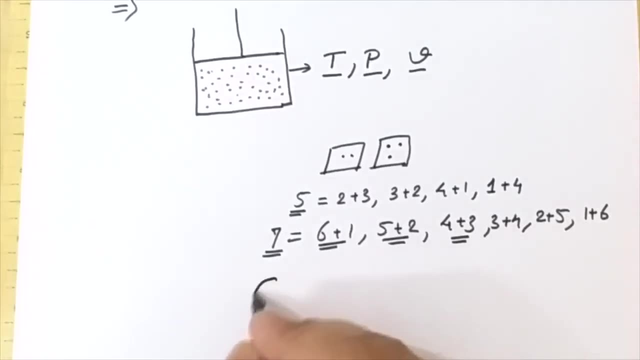 macrostate, it remains same, okay. similarly, i will give you one more example. that is, we are having a coin and in coin, or if we are having two points and in two points. if i want one head and one tail, so one hand, one head, that is, i want one head and one tail, so the possible combination is that coin. 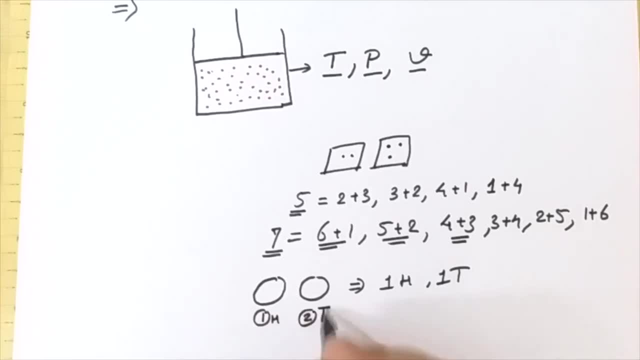 number one will give me head and coin number two will give me tail. or coin number one will give me tail and coin number two will give me head. so these are the two possibilities by which i can get head and tail. so our macro system. so these are our macro systems and this is our micro system. so 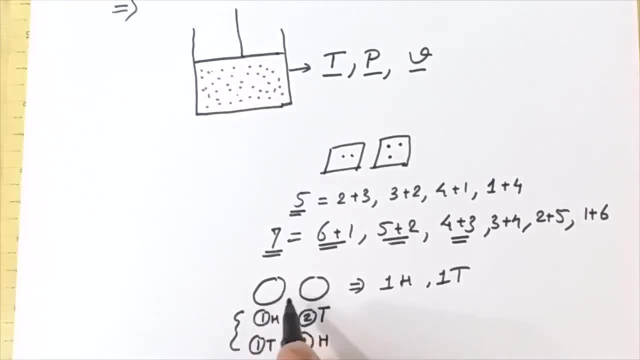 irrespective of the micro systems, our macro system remains same. so in this way we can say that micro system is- or sorry, the microstate is nothing, but it is the internal arrangement of the particle in the system and the property which is arised because of that internal arrangement, or the properties arising due to that, is known as macro state. okay, 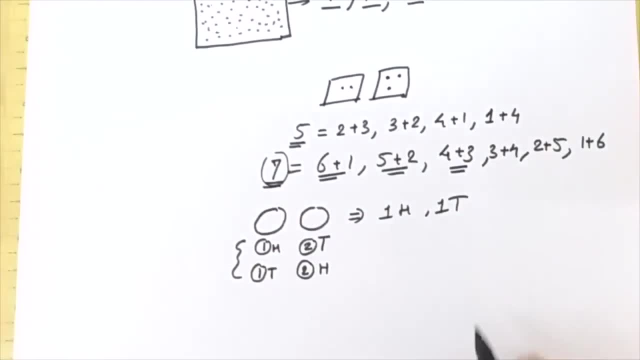 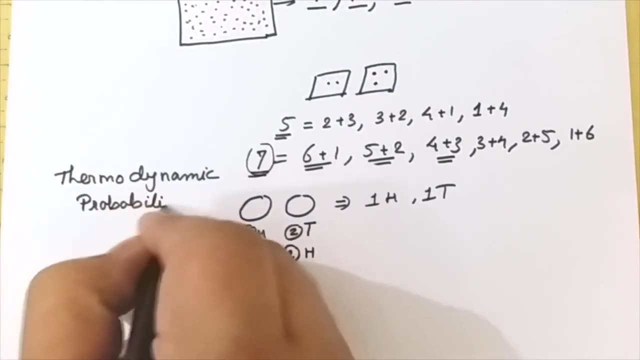 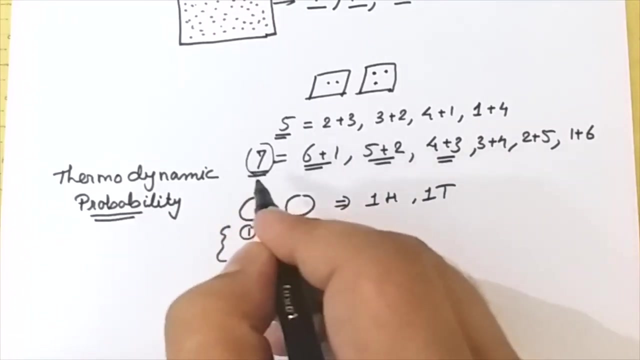 and there is one more definition, or there is one more property that is coming into picture and that is known as thermodynamic probability. so it is thermodynamic probability and this thermodynamic probability is nothing, but it is, it can be defined. as for a given macro state, how many different? 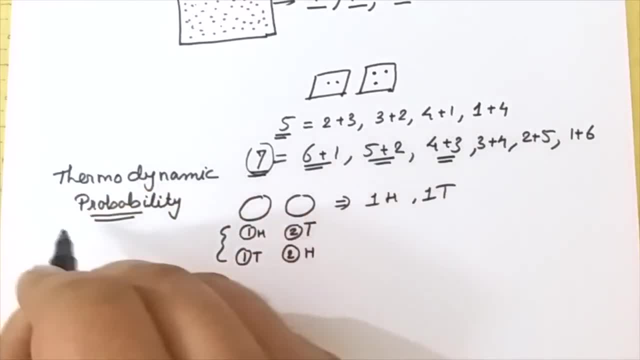 microstates are possible. so for a given macro state, how many different microstates are possible. it is known as thermodynamic probability. so again, take the example of seven. so seven can be obtained by one, two, three, four, five and six methods. so over here for micros. for 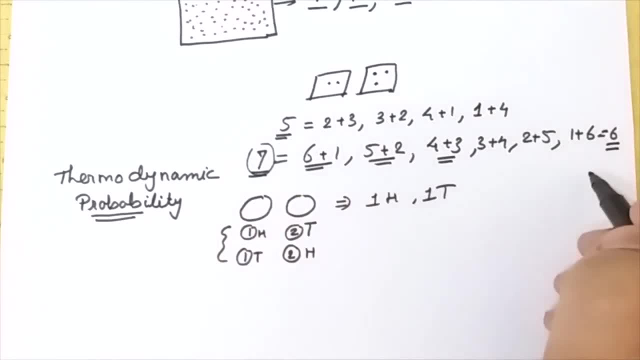 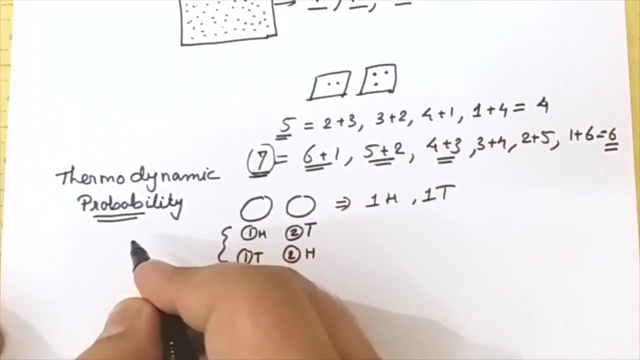 macro state seven, the thermodynamic probability will be six. that is, by six different ways we can obtain seven. similarly, for five, the thermodynamic probability is four. so by four different ways we can obtain five. so thermodynamic probability is nothing, but it can be defined. as for a macro state, 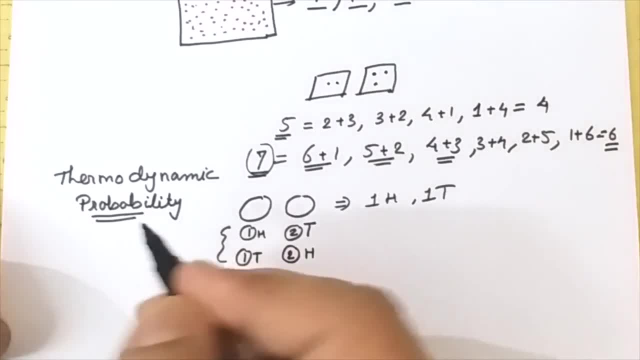 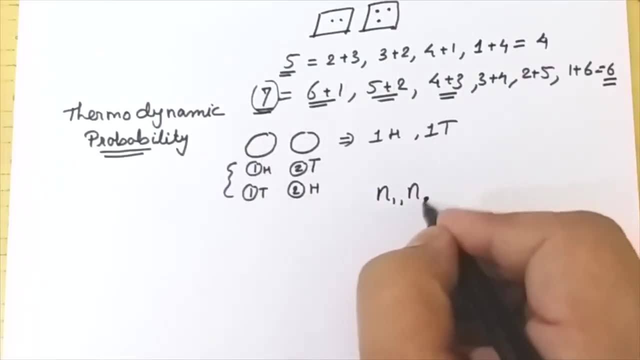 how many total number of different ways a micro state can be realized or micro state can be obtained. now suppose we consider that we are. we are having n1, n2, n3 and up to an n number of particles and these particles are arranged in n1, n2, n3. that is, n1 will go in n1, n2 will go in n2, n3. 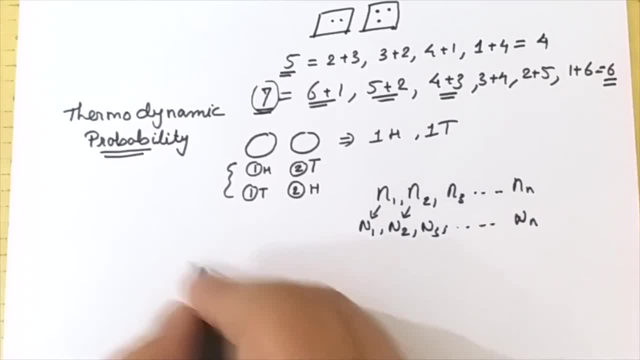 and so on up to an end. so the thermodynamic probability, and this thermodynamic probability is represented by w. so thermodynamic probability, w, it is given by, we can say n factorial upon n1 at capital, n. so n1 plus n2, up to sorry, n1 factorial into n2, factorial up to